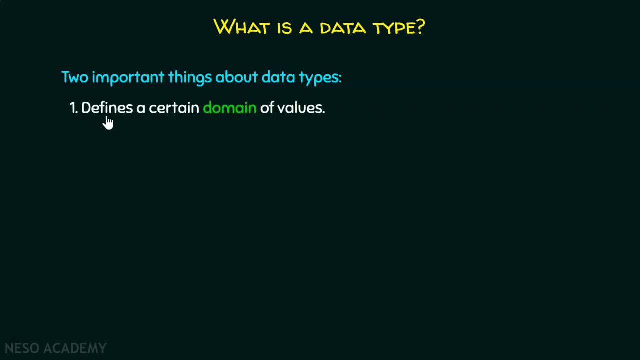 which I haven't told about data types, First is it defines a certain domain of values. We already know that a data type defines a certain domain of values, But there is one more important point, which says that it defines operations allowed on those values. 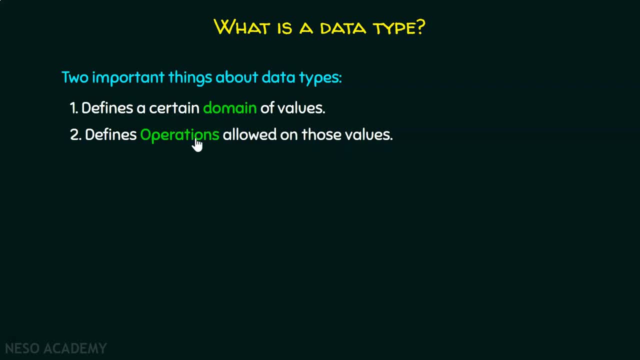 So not only it is defining certain domain of values, but it also defines what operations are allowed on those values. For example, we can think of integer type. Here we can take only integer values. We already know that integer allows only integer values. 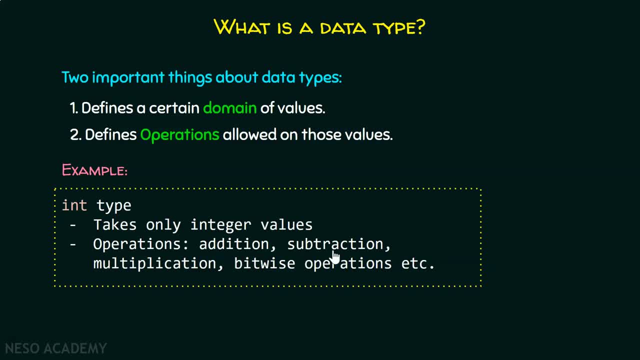 But the operations allowed are addition, subtraction, multiplication, bitwise operations, etc. We can perform almost every operation with integer type. For the sake of understanding, let's take another type, that is float type. It takes only floating point values. We already know that the domain of values 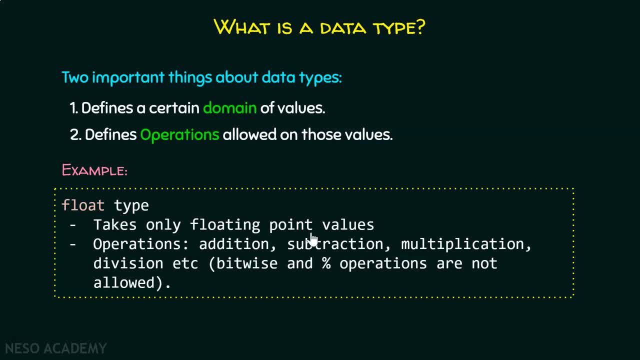 allowed in the case of float type are only floating point values. But the operations which we can perform on float types are addition, subtraction, multiplication, division, but we cannot perform bitwise and mod operations on them. This should be well noted. It is clearly understandable that. 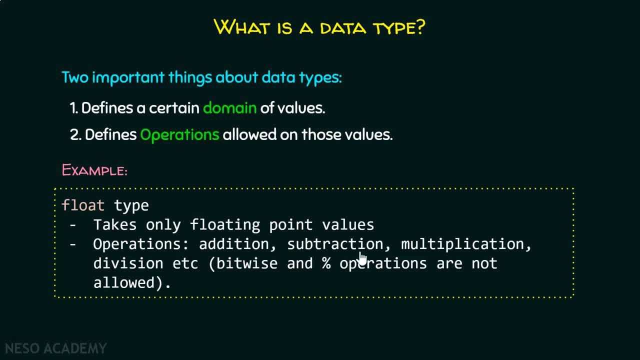 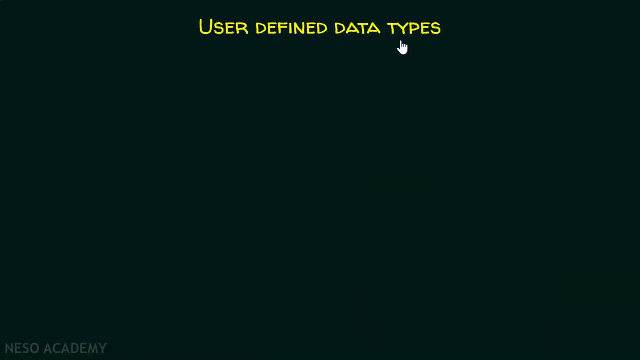 a data type not only defines a certain domain of values, but it also defines operations allowed on those values. Now let's discuss what is a user defined data type. Before moving on to abstract data types, we should understand what is a user defined data type. 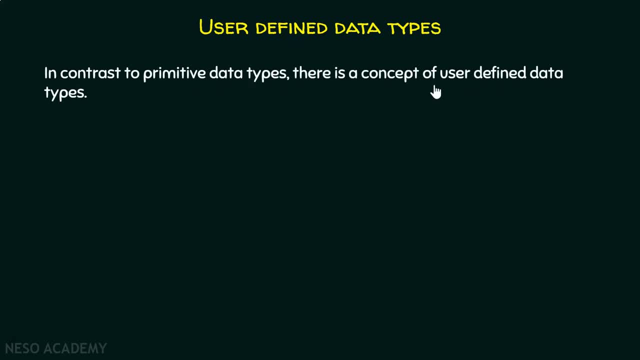 In contrast to primitive data types, there is a concept of user defined data types. We already know primitive data types, like integer, character float, But there is a concept of user defined data type which we should also know The operations and values of. 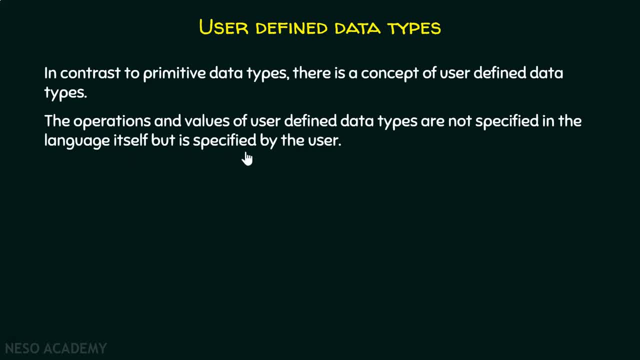 user defined data types are not specified in the language itself, but is specified by the user. Here the user is defining the operations as well as the values. It is not predefined in the language itself. Now here are the examples: Structure, union and enumeration. 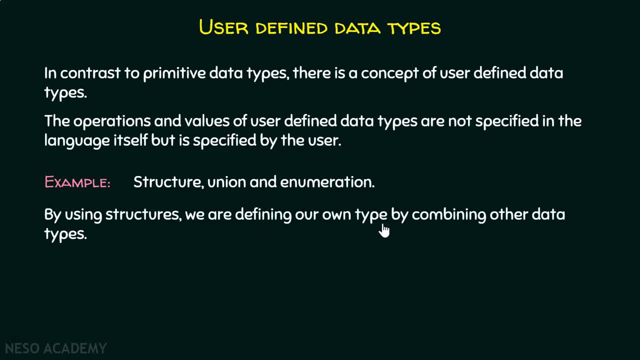 which we have already discussed. By using structures, we are defining our own type by combining other data types. By using structures, we are defining our own type by combining other primitive types, For example here, in this case, we have combined these two integers. 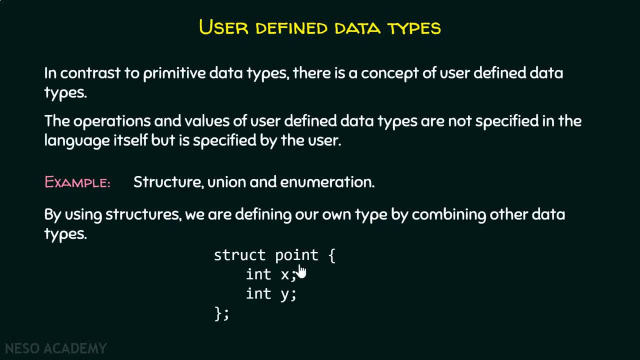 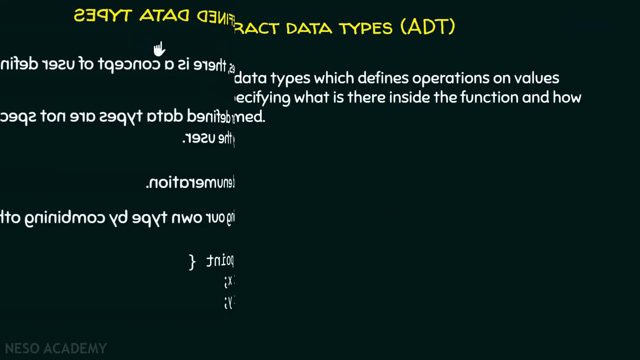 to form a new type. that is point. So it is a user defined data type. This is our understanding about user defined data types. Now let's try to understand what are abstract data types. ADTs or abstract data types are like user defined data types. 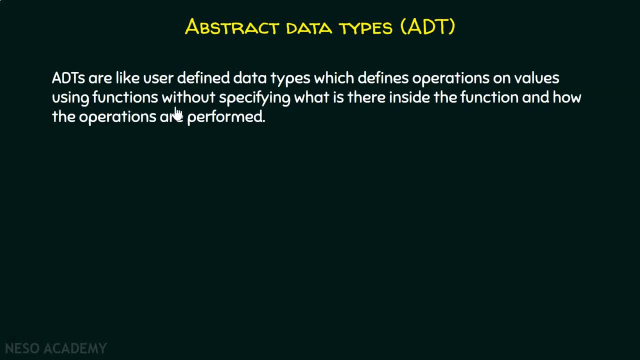 which defines operations on values using functions, without specifying what is there inside the function and how the operations are performed. First of all, we are defining operations- that is true, but we are defining operations on values- that is also true- using functions. It should be well noted that 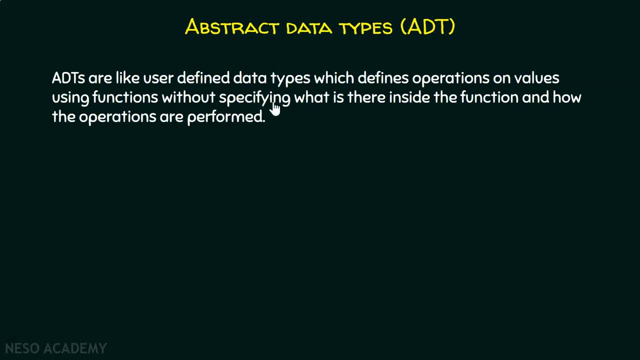 we are defining operations using functions without specifying what is there inside the function. We are not specifying anything inside: what is there inside the function And how the operations are performed. Let's take an example of a stack ADT. A stack consists of elements: 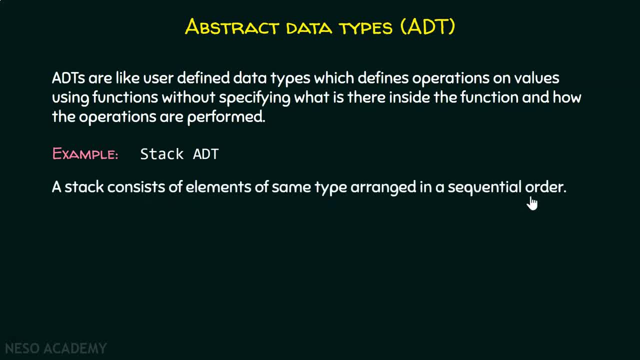 of same type, arranged in a sequential order. So what type of elements are allowed in a stack? The elements of same type, And that too, they are arranged in a sequential order. We already know that, right Now, the operations allowed on them could be: 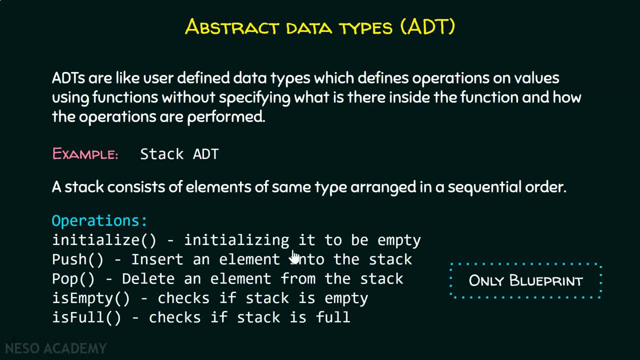 initialize. we can define an initialize function which initializes the stack to be empty. actually, We can perform a push operation, that is, insert an element into the stack. We can perform pop operation, that is, delete an element from the stack. We can check: is stack empty? 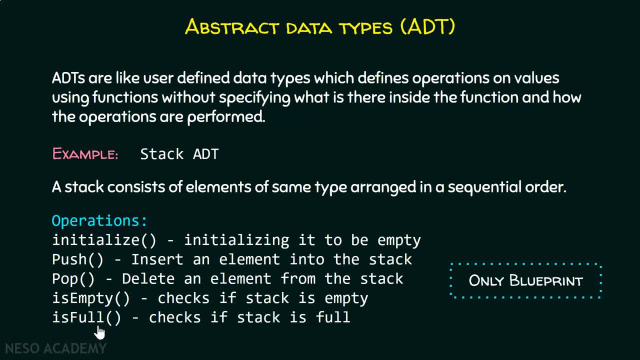 or we can check, is stack full? So these are the operations which we can define. These are functions. as you can see, Here we are specifying functions, but we are not saying anything how they can be implemented. We are just specifying them. That is called abstract data type. 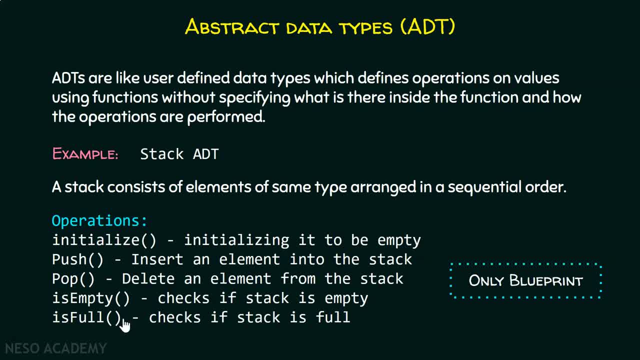 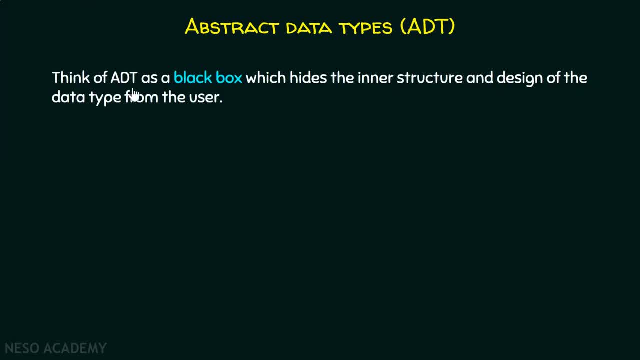 We know that what type of elements are allowed, and we also know that what operations we can perform, but we don't know what is there inside. Okay, Think of ADT as a black box which hides the inner structure and design of the data type from the user. 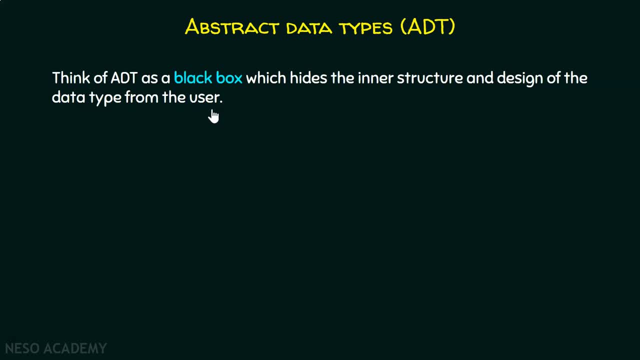 We can think of it like: it hides all the implementation details from us. This is very important, which we will understand later. There are multiple ways to implement an ADT. Let me tell you this is very important. There are multiple ways to implement an ADT. 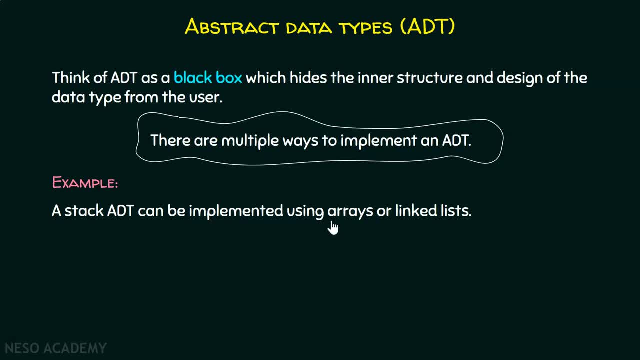 For example, a stack ADT can be implemented using arrays or linked lists. It should be well noted that stack itself is a data structure. We can implement this data structure using other data structures like arrays or linked lists. So a stack ADT, which we know, 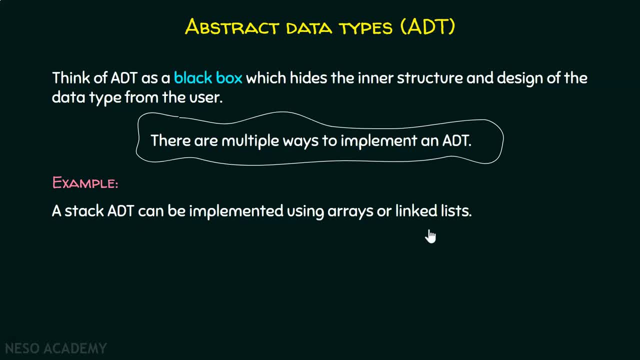 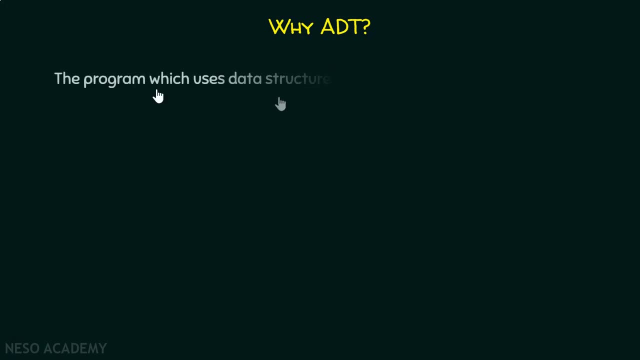 can be implemented using arrays or linked lists. Now the question that immediately arises that why do we even need ADTs? Why do we need skeletons? Why can't we simply implement things displayed to the user? Why ADT Before moving further? 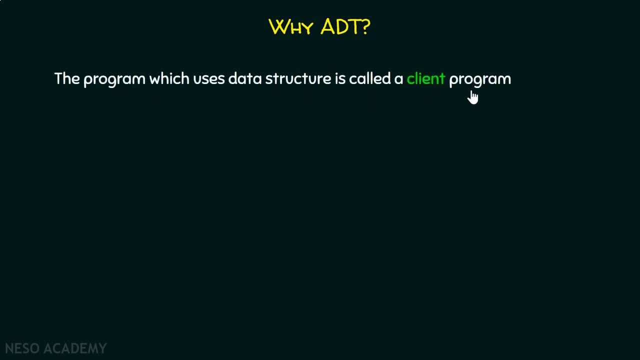 we should understand some terminology. The program which uses data structure is called a client program. You should note this very clearly: that the program which uses data structure is called a client program- Nothing else, just abstract- And the program which implements the data structure is called implementation. 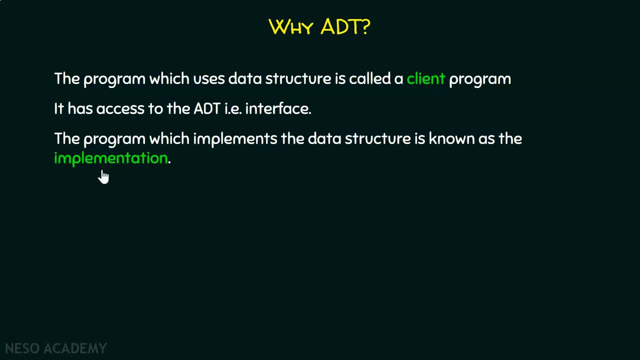 So we have two programs. One is client program and the other one is implementation. Implementation is the one which implements the data structure, and the client program is the one which just uses the interface. That is the outside details, nothing inside. Now let's discuss the advantage. 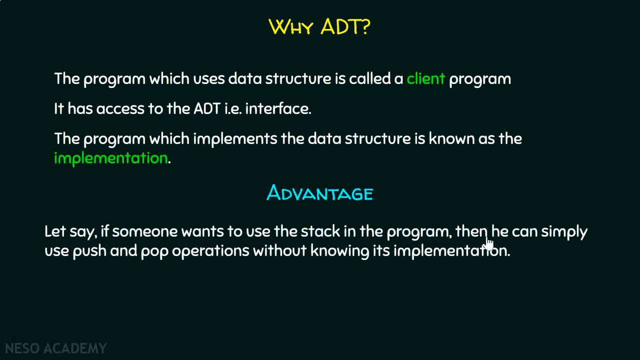 Let's say, if someone wants to use the stack in the program, then he can simply use push and pop operations without knowing its implementation. A user doesn't have to worry about how the operations are performed. Okay, If someone wants to use the stack program. 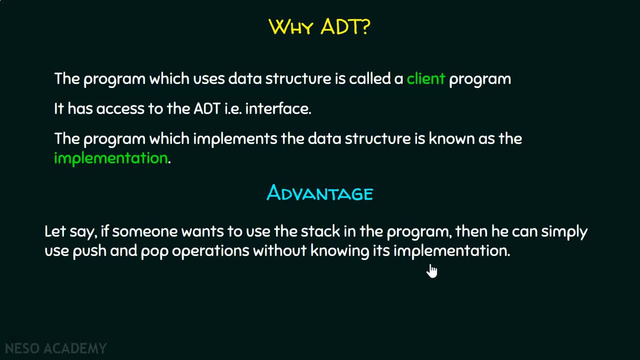 we know that the program which uses the data structure is called the client program. It has access to the interface only and nothing inside, So he can simply use push and pop operations without knowing its implementation. Apart from this, if in future the implementation of stack is changed, 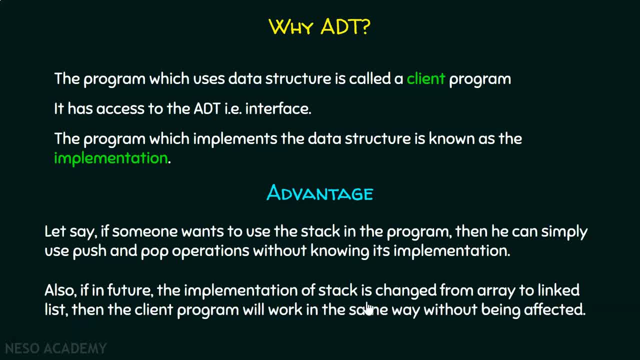 from array to linked list. let's say, previously the stack was implemented using arrays, right, But now let's say it is changed to linked list, The client program will work in the same way without being affected. There is nothing to discuss with client program. 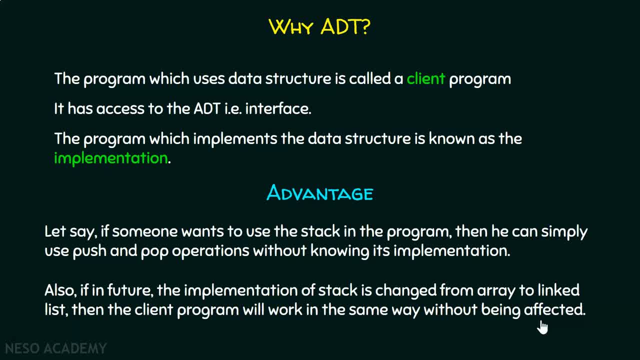 Client program has nothing to do with it. It can simply use the interface without knowing what is going inside. So if the implementation is changed from array to linked list, nothing will be affected in the client program. This is one of the biggest advantages.